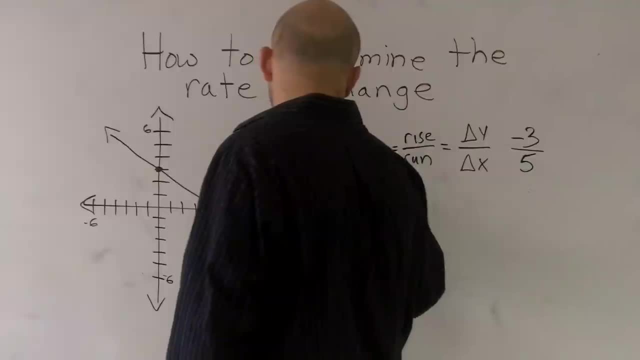 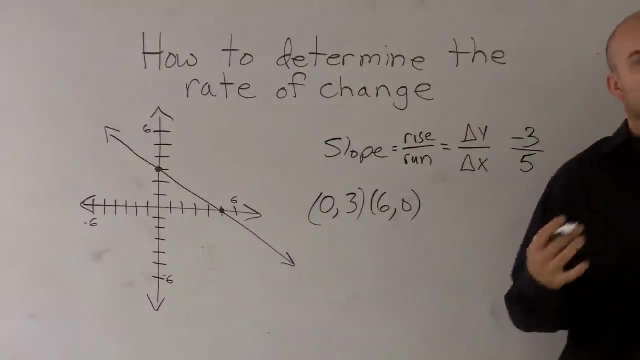 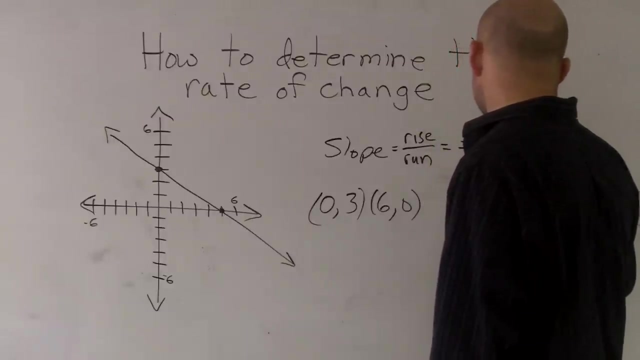 let's say this is at 0.03, and this is at 0.60.. So if you guys remember the slope formula, which is that delta y over delta x is written as this: m equals y2 minus y1 all over x2 minus. 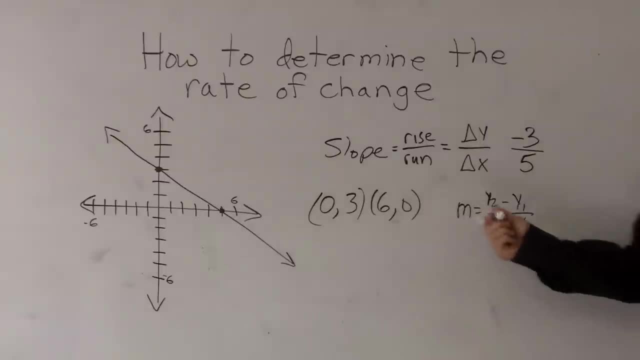 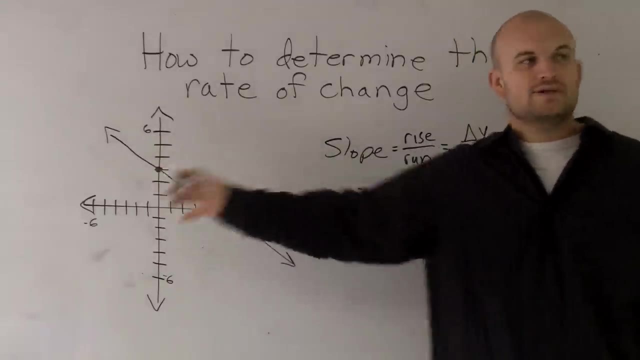 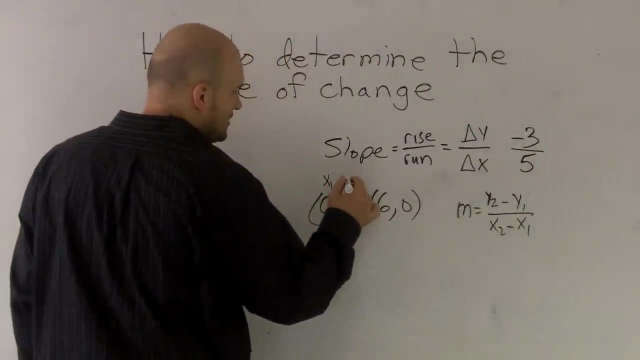 x1.. So therefore, now, what I can do is, if it's hard for me to determine- I can't count on a grid, I can't see it- I can always transfer two points into coordinate form and then use my slope formula to solve the rest. So here this is actually going to be pretty easy. 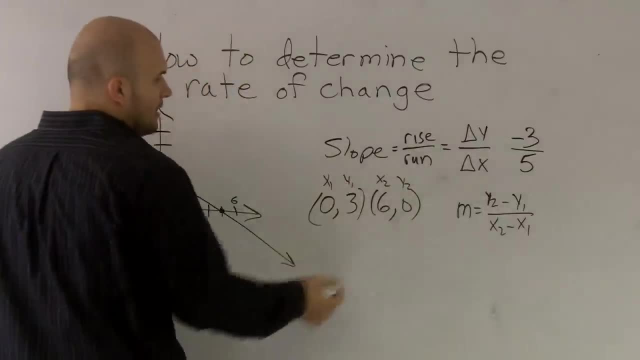 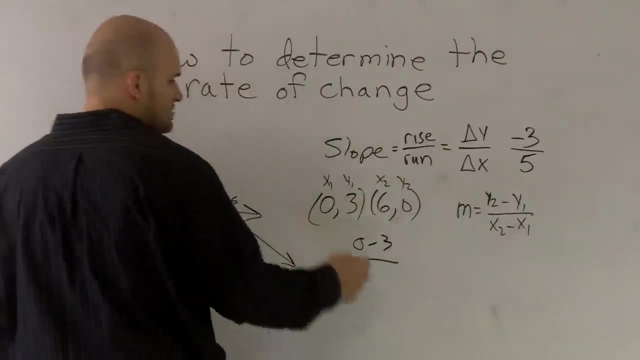 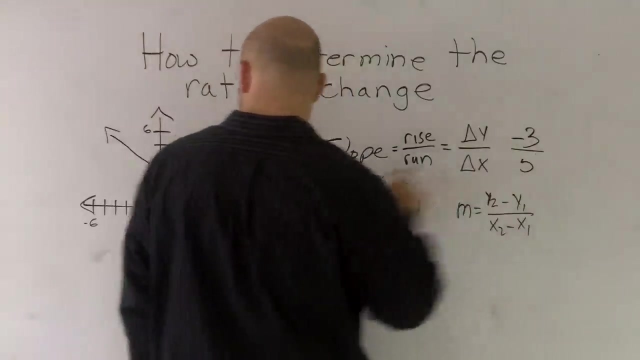 I'm going to label these x1, y1, x2, y2, and then just simply solve: So 0 minus 3, all over 6 minus 0.. OK, when did I? when did I? why is that 6?? That's supposed to be a 5, isn't it? 1,, 2,. 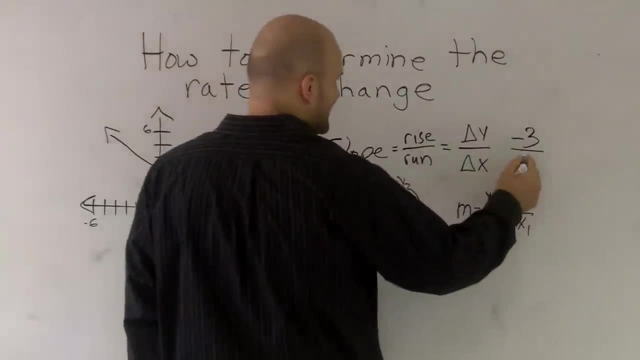 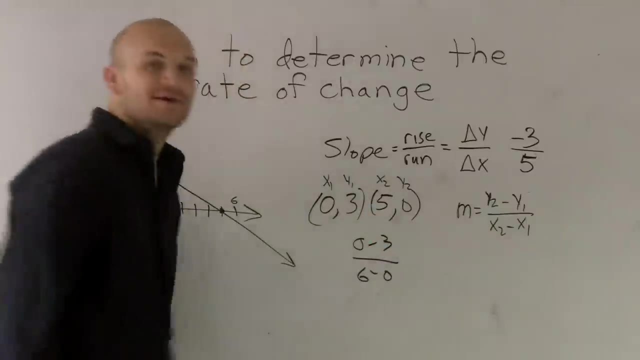 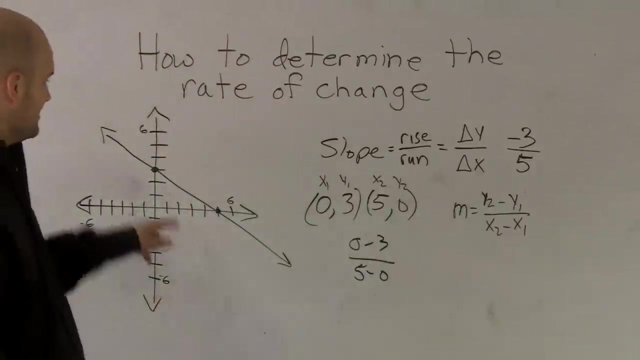 3, 4.. Oh no, that's not 6.. OK, that is a 5.. My bad, Your 0.2 is not at 6,, it's at 0, at 5.. My apologies, So this is going to be a 5.. I was seeing a 6, and that's what I was thinking. 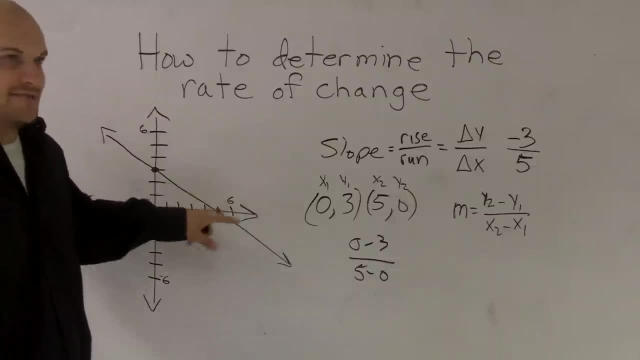 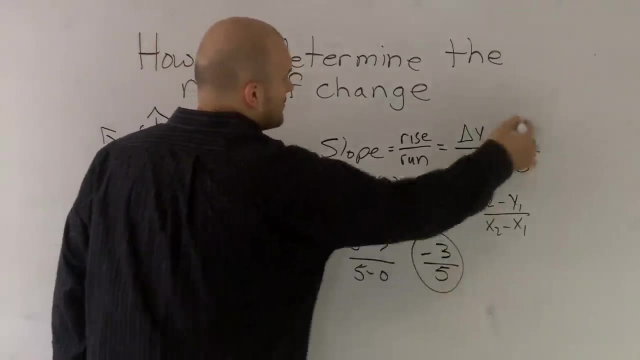 Your intercept's at 5,, not a 6.. 6 was my scaling, So 0 minus 3 is a negative 3.. 5 minus 0 is 5. And therefore you guys can use either method to go ahead and solve. So that's how you determine. the rate of change when given a graph or when given two points.